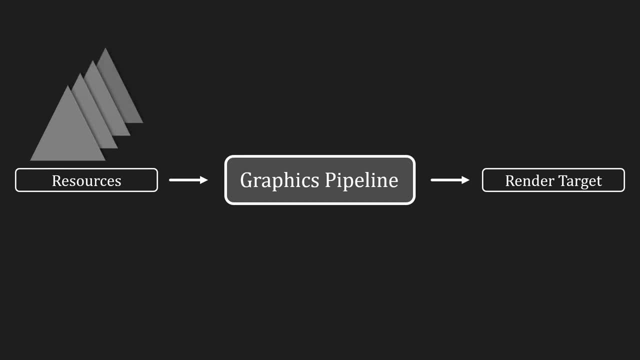 The resources are triangles which make up a 3D model, as well as textures. The output is the final rendered model. So the question is: what goes into the graphics pipeline to transform these triangles and textures into a rendered model, And there is multiple different stages. 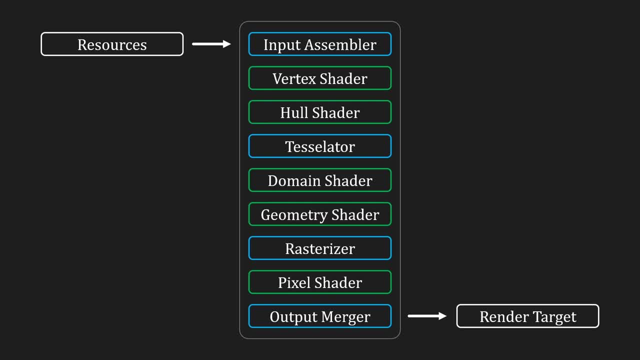 We're gonna go over all of them, but for now I want to focus on the fact that some of them are blue and some of them are green. The blue ones are fixed function stages, which means that we can set a few parameters to define their behavior, but that's all the control we have here. 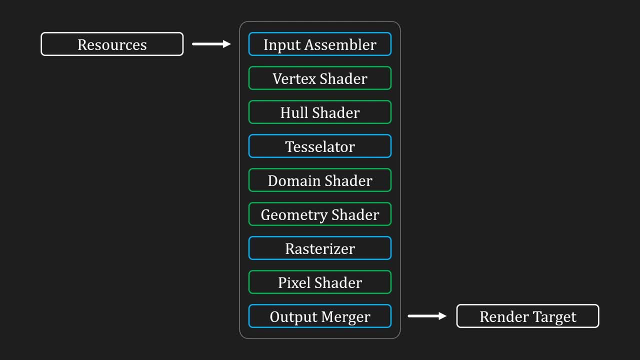 The green ones all end in the word shader, and a shader is a little program which we can write by ourselves and which runs on the graphics card. Since we can write code to define these stages, we have a lot of control over what they do. Let's get started with discussing the input assembler. 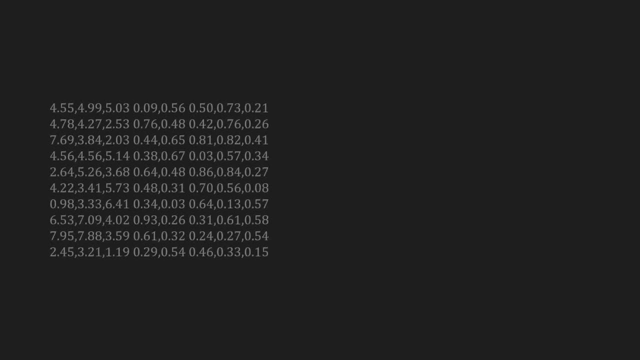 Its input is a vertex buffer which contains all the vertex attributes for every triangle that makes up a 3D model. Example 1: The product has a code which marks what the graphics data will look like. It will be a vertex buffer that contains all the vertices which will be used for the purchase of the. 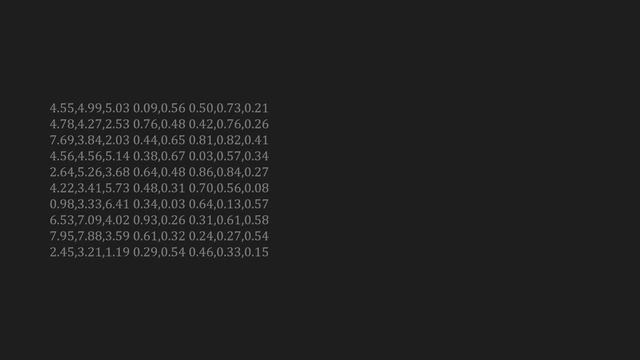 Problem is that, since all of this data is in one big chunk of memory, we can't distinguish the individual attributes. Therefore, we have to tell the input assembler which attributes make up a vertex. For example, for this vertex buffer, we have a position, a UV coordinate and some normals. 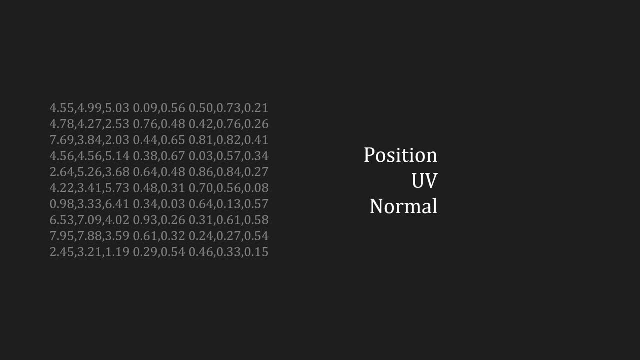 This data is not enough, though. We also have to specify how many components make up the vector that defines these attributes. For example, the position is a three-dimensional vector, the UV coordinate a two-dimensional vector and the normal a three-dimensional vector. 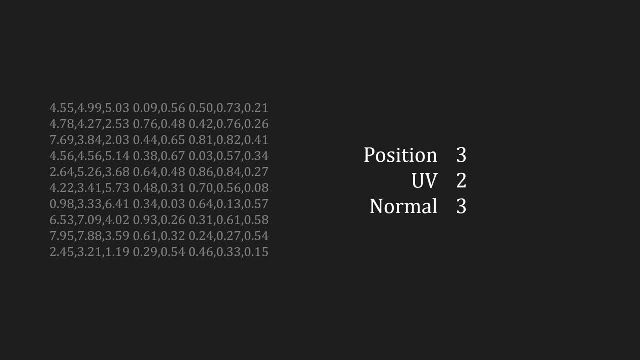 You might be thinking that it is redundant to specify the amount of components that make up a single attribute. however, in the case of a position, you could, for example, also have a two-dimensional position, or, in the case of a normal, you could use polar coordinates. 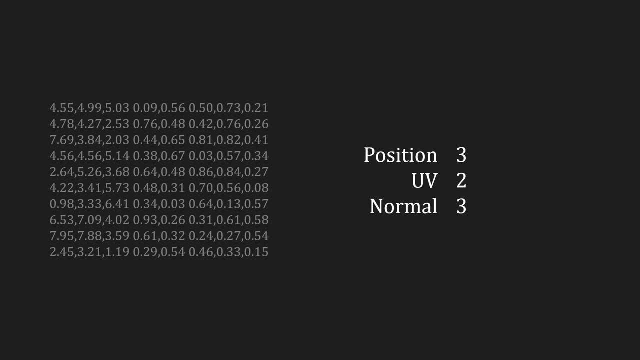 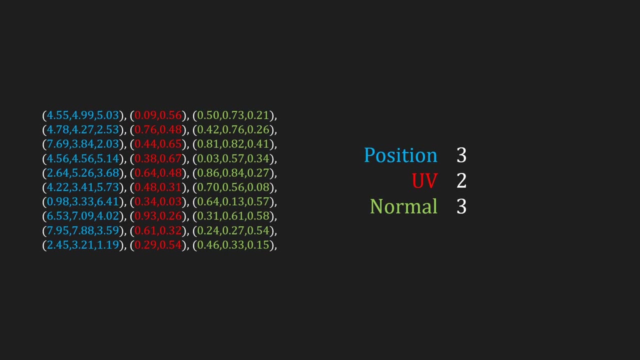 to pack it into two components. With this information, we are now able to distinguish the two-dimensional vector. The problem is that a computer needs a bit more information, since it won't store the numbers in decimal form like I've written them here. instead, it will store them as. 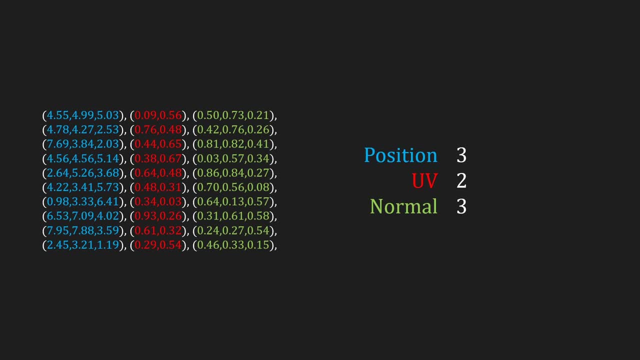 binary numbers, which means it has to know which format it has to use to convert them back to decimal numbers. In this case, all the components could get stored in a floating-point number of 32 bits. Once again, that's a little implementation detail. 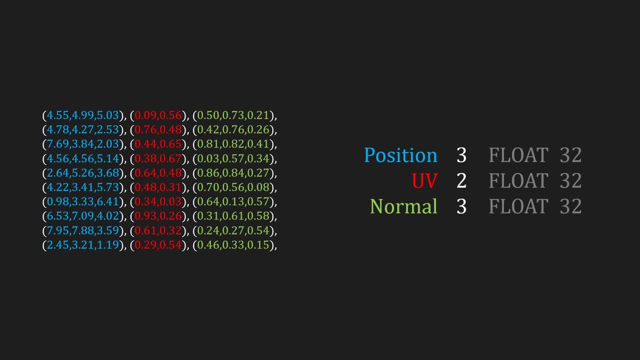 That is not really of importance to us. The input assembler can also assign extra vertex attributes, for example a vertex ID which starts at 0 and increments to however many vertices there are. The ID takes up one component and gets stored as an unsigned integer, probably of 16 bits. 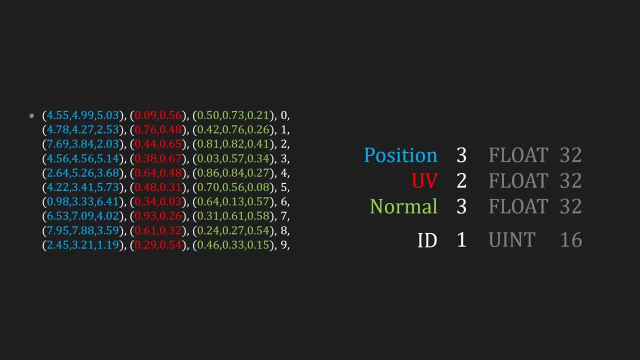 Every row in our vertex buffer now represents a single vertex, and every single vertex in the vertex buffer will now get passed on to the vertex buffer. The vertex buffer will now get passed on to the vertex buffer. The vertex buffer will now get passed on to the next stage, which is the vertex shader. 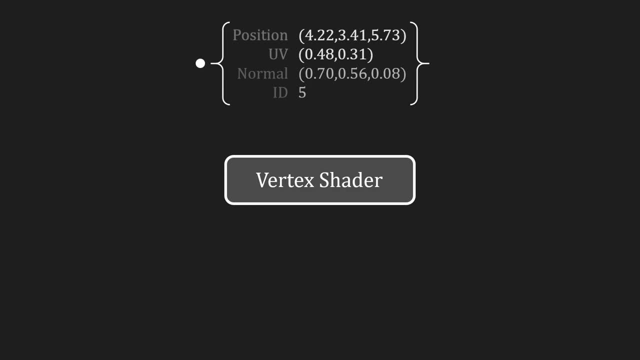 The vertex shader takes in all the attributes of a single vertex and outputs a new set of attributes. To do that, it will use some external data, for example a matrix. We'll discuss those in detail in a future video, but for now, all you have to know is: 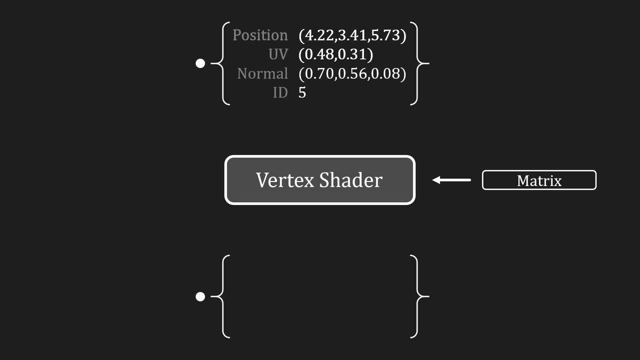 that we can multiply the position with a matrix to transform the position. So when the position goes into the vertex shader, it comes out as a different vector, A vector that is transformed by the matrix. The vertex shader can also just pass attributes without modifying them. 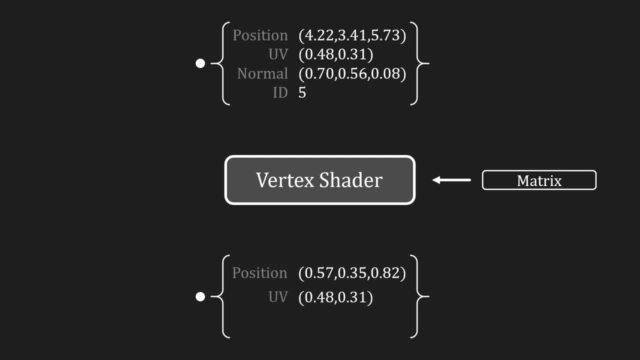 For example, the UV coordinate usually just gets passed, Or it could also introduce new attributes, For example this color attribute: Every single vertex that the vertex shader outputs should have a position that is in a row range between negative 1 and 1.. That means that every vertex that exits the vertex shader 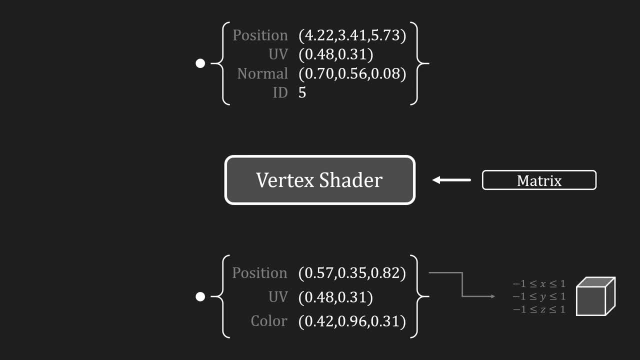 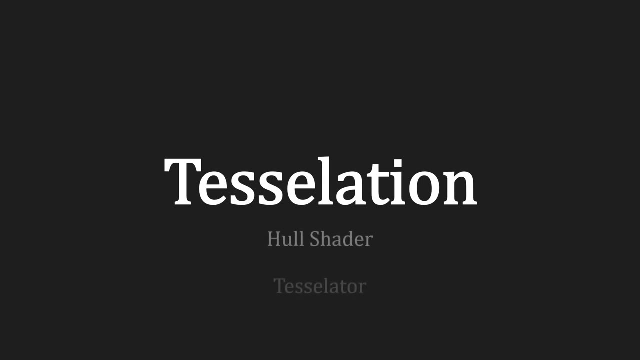 ends up in a cube of 2 by 2 by 2.. For programmers who are watching these videos, here's the code of the vertex shader I just described. The next stage in the pipeline is the tessellation stage, which is a combinational name for the hull shader, the tessellator. 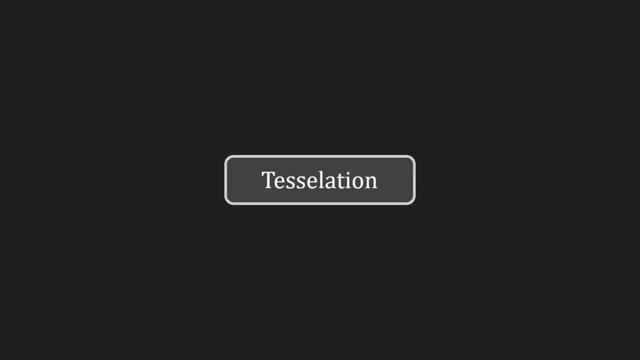 and the domain shader. The tessellation stage takes in a primitive, for example this square, and it outputs a more detailed version of its input. In other words, the output contains more triangles. Tessellation is a rather advanced topic, so I won't cover it in depth here. In short, though, the way it works is that the hull shader 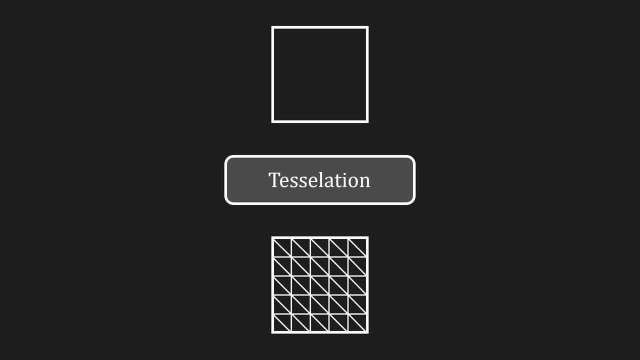 defines the pattern for the output triangles. The tessellator will then create those triangles based on that pattern and then it will be displayed in the case. domain shader will then position the triangles based on some formulas. A potential use case for tessellation is taking in a low-poly model and outputting a high-poly model by introducing 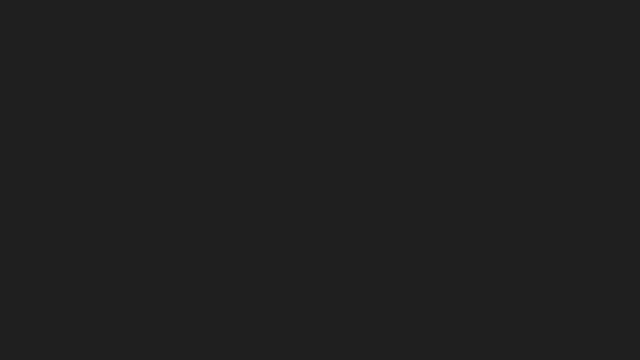 more triangles. The next stage in the graphics pipeline is the geometry shader. It takes in an entire primitive which is a triangle and additionally it can also take in the adjacent vertices to that triangle and it outputs a modified version of its input, For example: 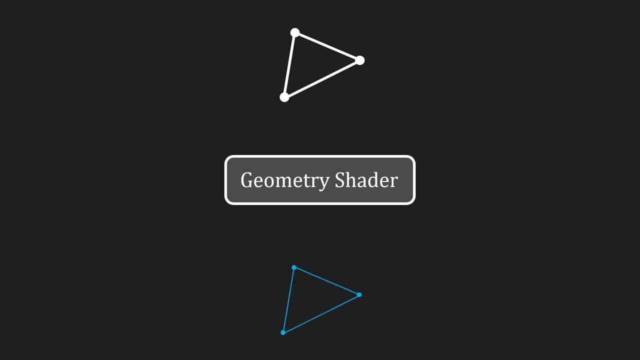 it could just output its input, but it could also introduce a new vertex which then turns this triangle into a pyramid. The primitives that enter the geometry shader don't have to be triangles, They could also be lines. The geometry shader now can take that line and expand it into. 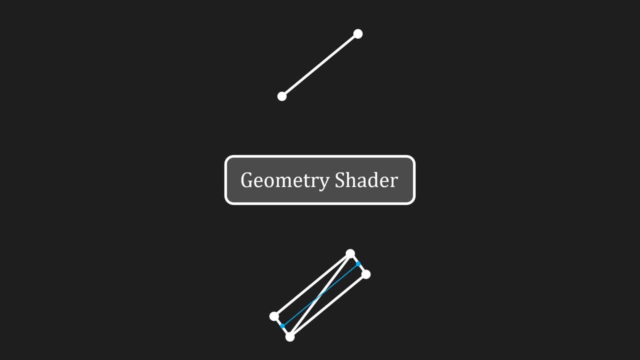 two triangles. This is useful when we want to modify the geometry shader. We can define the hair as a line, but since a line doesn't have a surface, we need a geometry shader to create that surface. One last primitive: we can enter into a geometry. 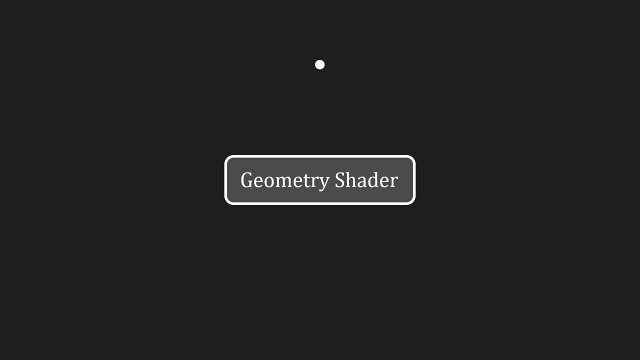 shader is a single point and the geometry shader can take that point and turn it into a quad. This is, for example, useful for particle systems. By now, the vertices have reached their final positions and it is time to draw them, and that gets done by. 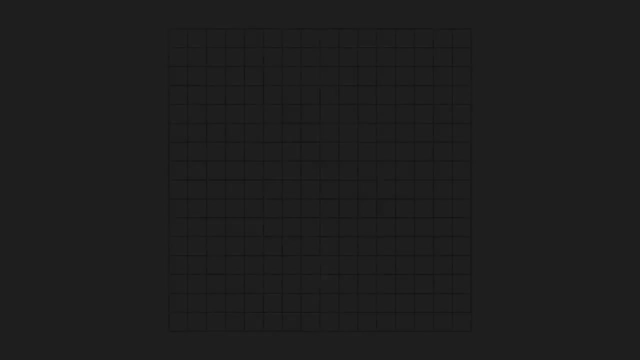 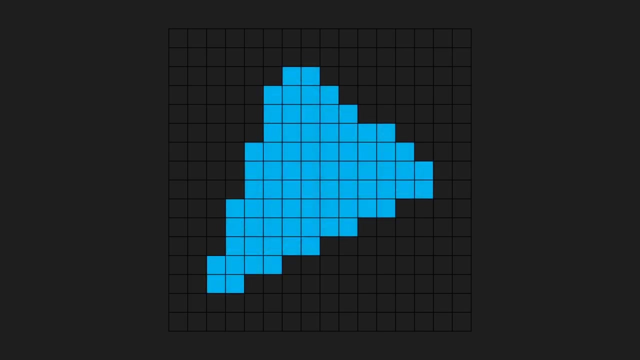 the rasterizer. The rasterizer outputs a grid of pixels and it takes in every single triangle, for example this blue triangle, and then it has to convert that triangle into a bunch of pixels, which would look like this: Now, the more pixels you have, of course, the better the approximation. 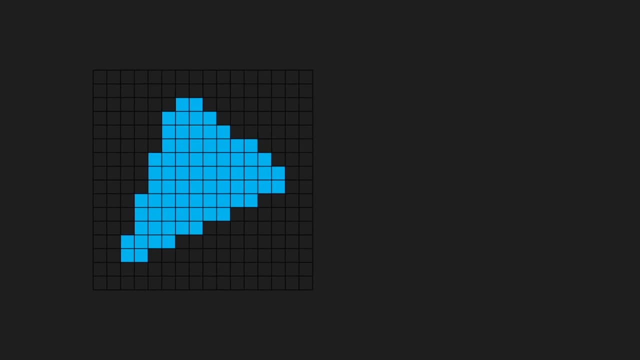 of the triangle. Let's have a look at the scene we just rendered. If this is the camera, then the camera obviously is the camera. If this is the camera, then the camera obviously is the camera. If this is the camera, then the camera obviously is the camera. 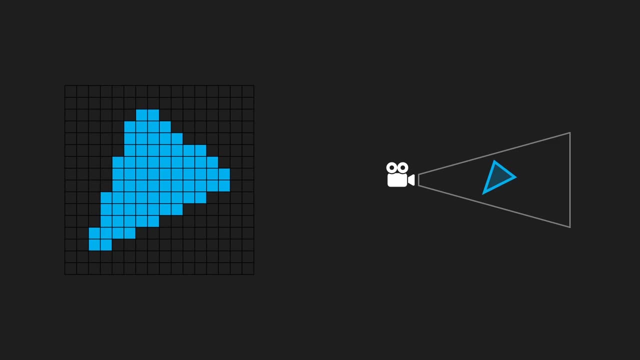 Now, what if there was also a red triangle behind the blue triangle? Well, the problem is that we already rasterized the blue triangle, So if we now also rasterize the red triangle, then it will appear in front of the blue triangle, which is, of course, wrong. Unfortunately, we can't solve this. 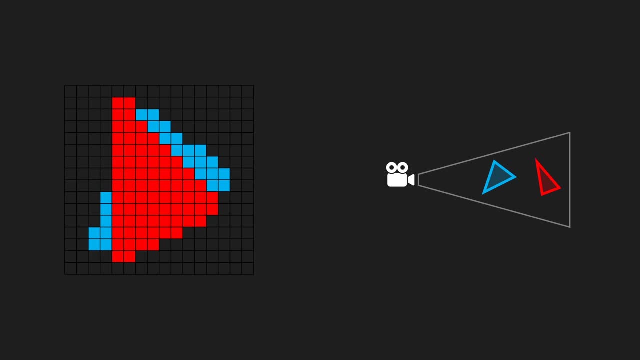 problem by changing the order in which we draw the triangles, since that is not possible on a graphics card. Unfortunately, we can't solve this problem by changing the order in which we draw the triangles, since that is not possible on a graphics card. The solution to our problem is to also use 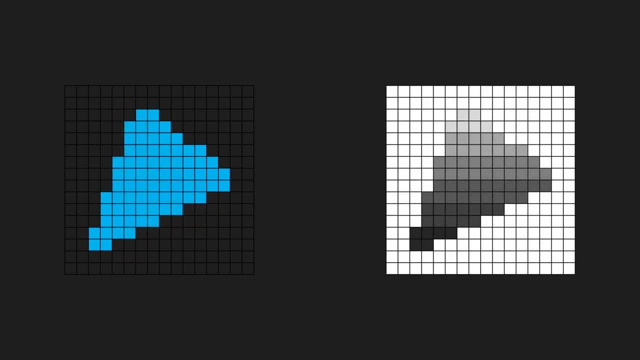 a second image, which we call the depth buffer or z-buffer. The way this image gets made is by converting the z-coordinate of a triangle's surface into a color. The closer the surface of the triangle is to the camera, the darker the color will be, In other words the bottom left. 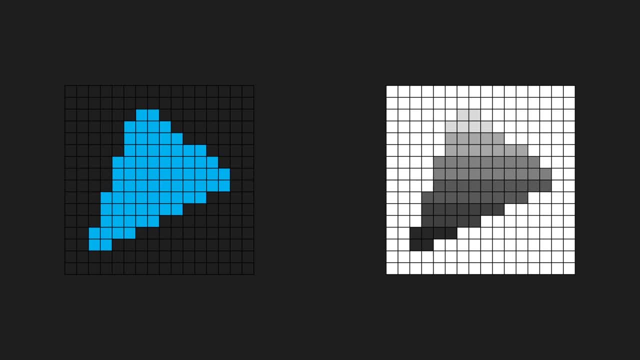 corner of the triangle is the closest to the camera. according to this z-buffer, If we now rasterize the red triangle, then only the parts that are behind the blue triangle will become visible And notice that we also write the z-values for our red triangle into the depth buffer. 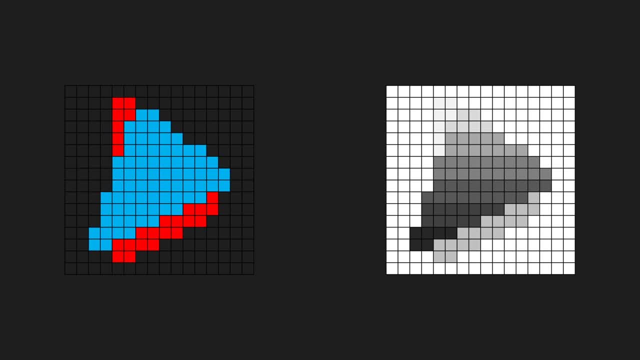 We'll come back to how and why this works in just a moment. For now, let's focus on the fact that our triangles only have a single color. What if we want to apply a texture to that triangle, for example? Well, the rasterizer is the stage which interpolates. 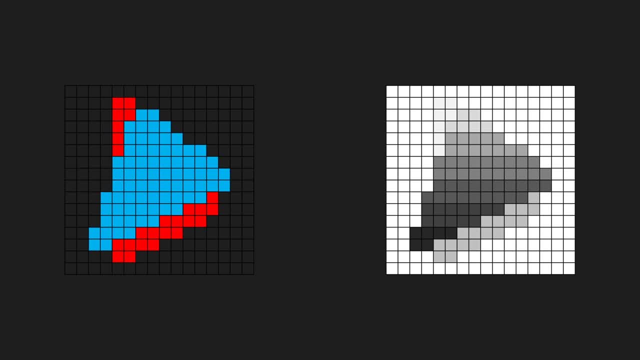 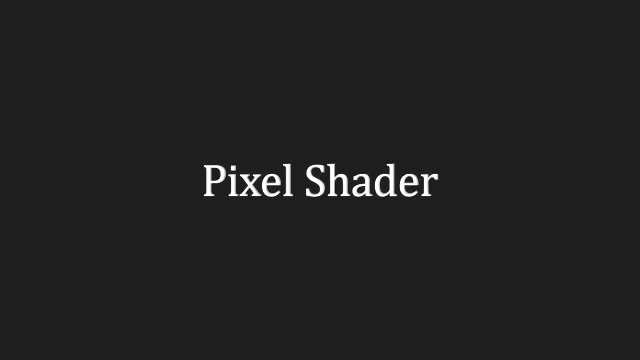 vertex attributes across a triangle's surface And for every pixel of a triangle it generates, it will pass those attributes onto the pixel shader, which is the stage that calculates the color. As I just said, the pixel shader takes in all the attributes of a single pixel and outputs. 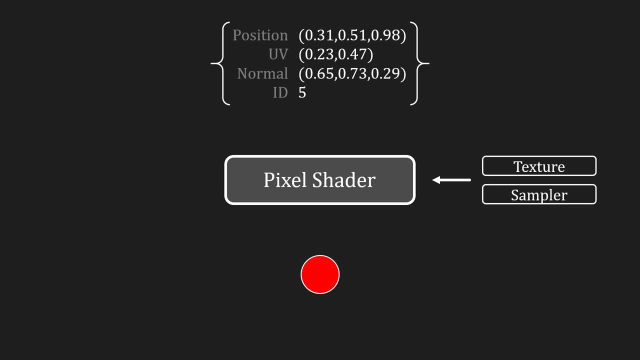 a color. It can do that based on a texture and a sampler. We discussed those in the last video, which I highly recommend you go watch. And for programmers, here's a code that assigns a color based on the UV coordinate, a texture and a sampler. The final stage in our graphics pipeline.